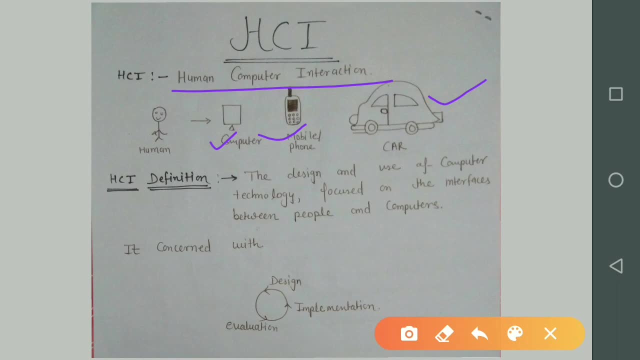 so many examples like calculator, alarm watch, etc. Computers are everywhere in our life. So what is the definition of SCI? First, the design and use of computer technology focused on the interfaces between people and computers In other way, and simple definition is in other way. 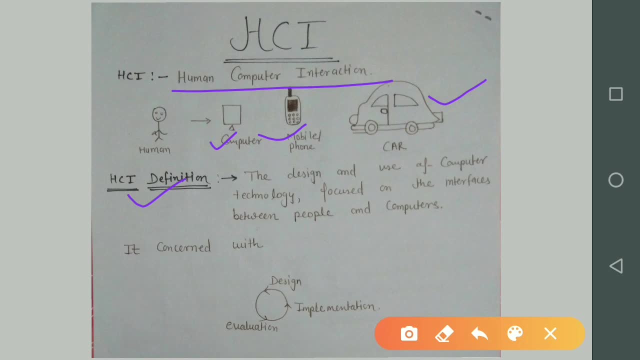 we can say interaction between human and computers, And SCI. it concerned with design, evaluation, implementation of computing system, we can say, which provides services for the human beings. There are so many examples of SCI. So what is the definition of SCI? First, the design. 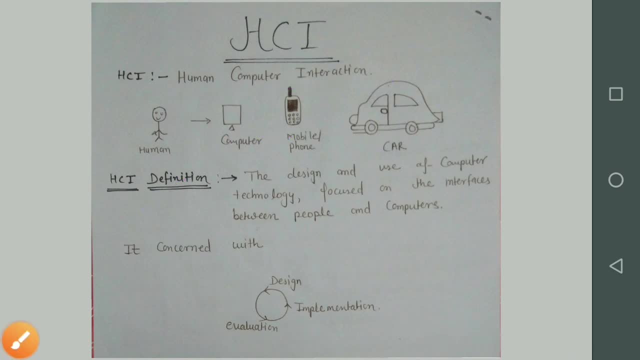 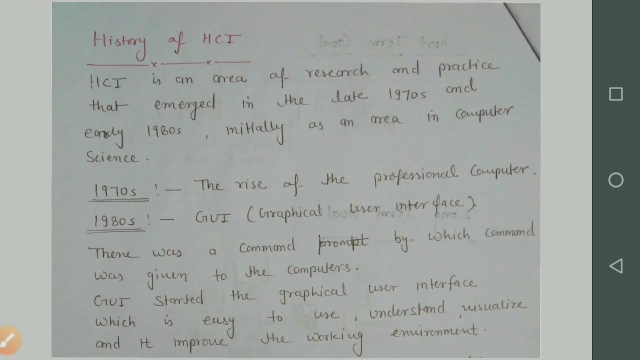 and use of computer, mobile phone and car. There are so many examples to interact with the computer system. So first of all, the history of SCI. SCI is an area of research and practice that emerged in the late 1970s and early 1980s, initially as an area in computer science. So in 1970s. 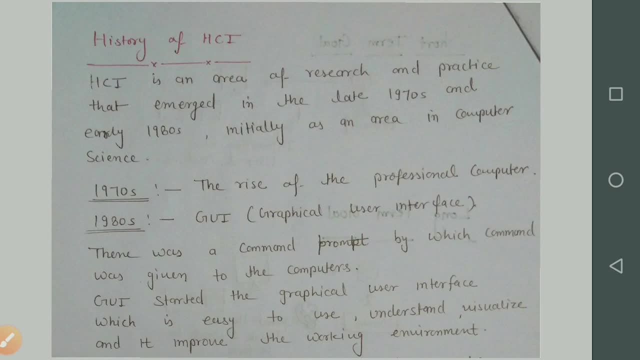 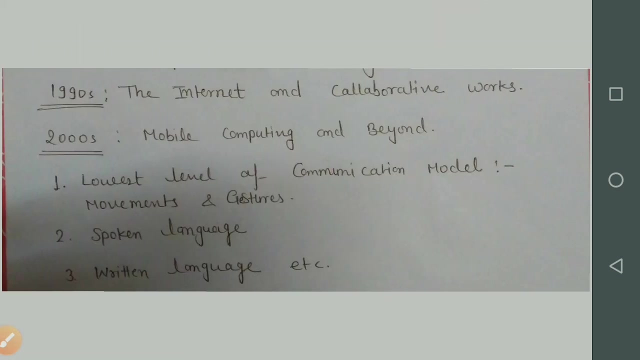 it used only professional computers In 1980s. GUI is there, So GUI is used to understand and visualize and it's improved the working environment. And after that in 1990, the internet and collaborative works. And last one is 2000,. mobile computing and beyond it. 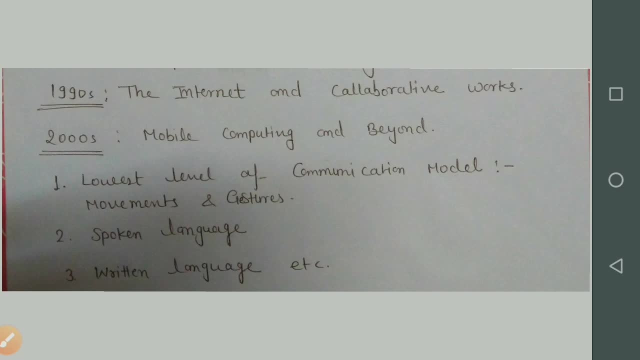 And after that there are so many ways to perform, to interact with the human, computer interaction or machine. So there are some interaction concepts. First is lowest level of communication models And it it is a movements and gestures, And these are language independent. So next is spoken language And after that written language. Now 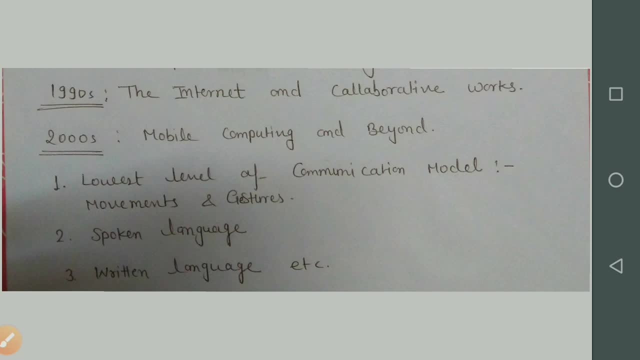 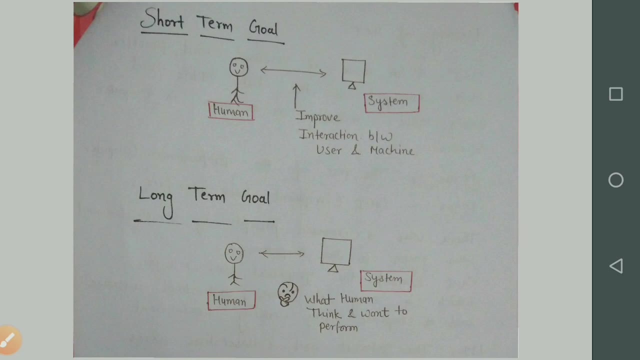 the modern time we have typewriters. there are so many methods to communicate with the machine. So after that we have two types of goal. There are short term goal and long term goal. Now the goal of SCI is to improve interaction between users and machines. 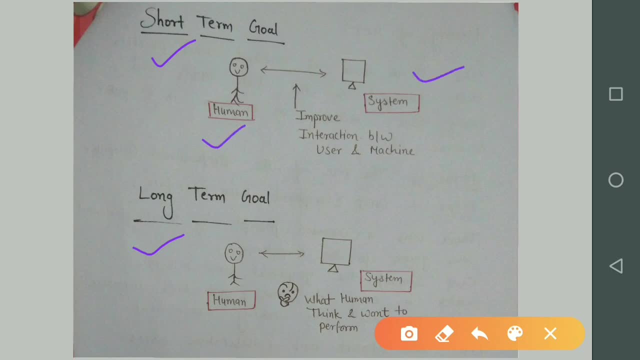 User and system. This is the short term goal. This is the short term goal, and our long term goal is to design the system that minimize the barrier between the woman's cognitive model of what they want, what they think, what they perform, what they want to do perform.